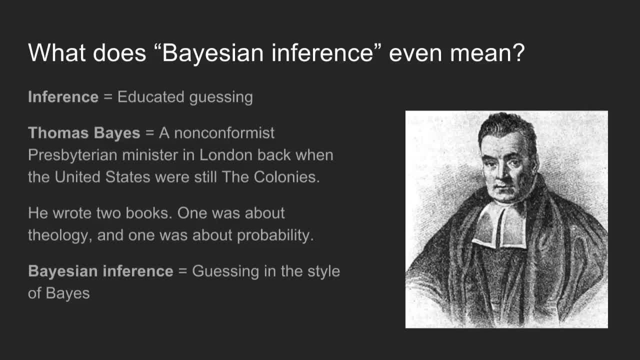 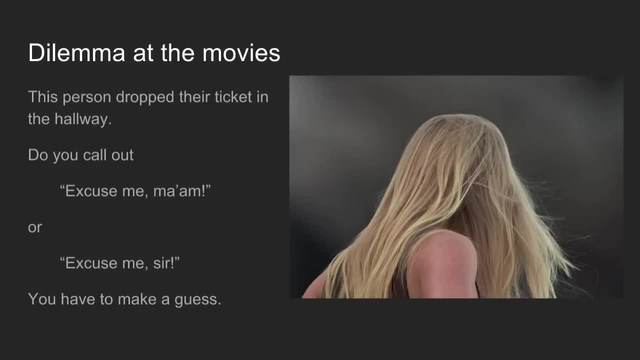 So Bayesian inference is just guessing in the style of Bayes. So to illustrate it, imagine that you're at the movies and someone drops a ticket. You pick it up and you can see them from behind. You know they have long hair, but 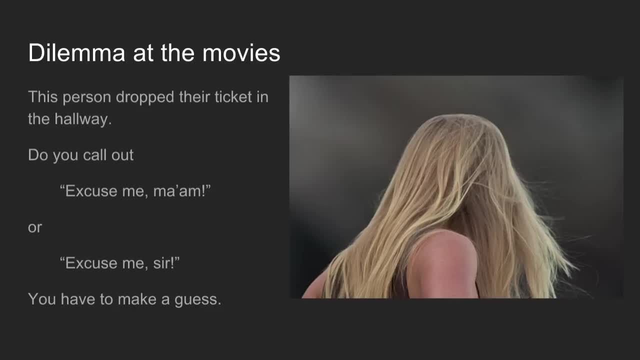 you don't know whether they're a man or a woman, so you have to make a guess Based on what you know about the attendees at your movie theater. you might say: excuse me, ma'am, is this your ticket? Now, imagine instead that this person is standing in line for the. 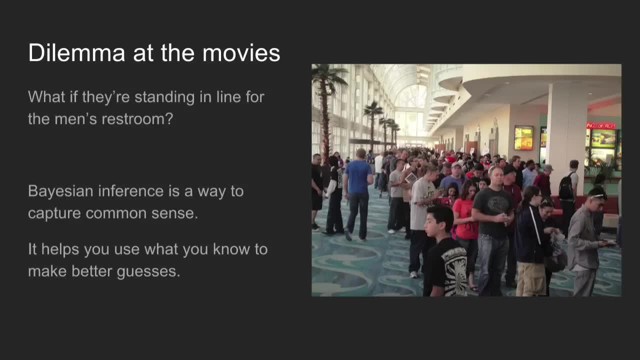 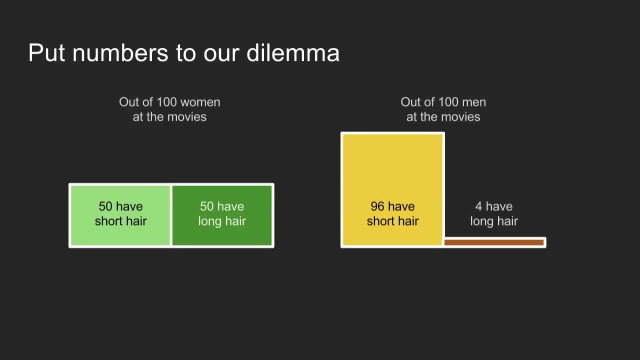 men's restroom. Knowing this extra piece of information, you might make a different guess. Okay, Bayesian inference is a way to capture this common sense knowledge about the situation and help you to make better guesses. So to put numbers to this dilemma, at the movie theater. 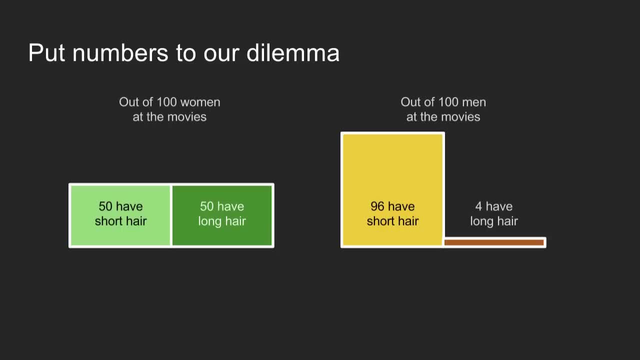 let's assume, out of 100 women at the movies, 50 have short hair, 50 have long, and out of 100 men at the movies, 96 have short hair and 4 have long. In this case we can see: 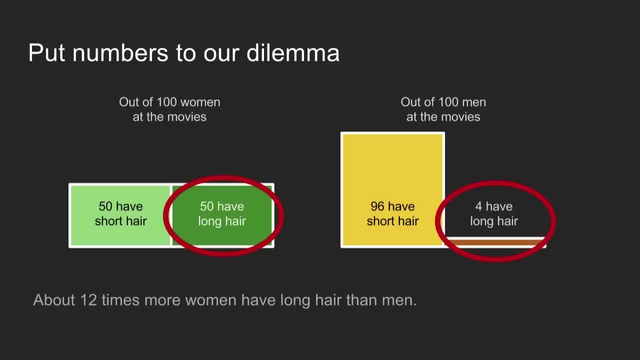 that there are definitely more women with long hair than men with long hair, so it's a safe bet to assume this person is a woman. Now, we just made a subtle assumption that there are about the same number of men and women at the movies. This assumption no longer. 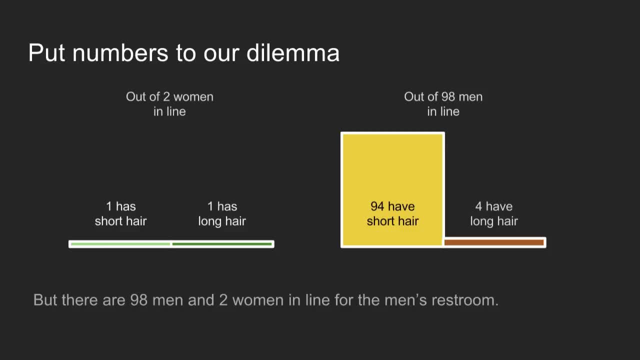 holds when we move to the men's restroom line. Here, let's say there are two women out of every 100 people and 98 men maybe. women keeping their partner's company. There's still one with short hair and one with long hair. There's still half and half with long and short hair. 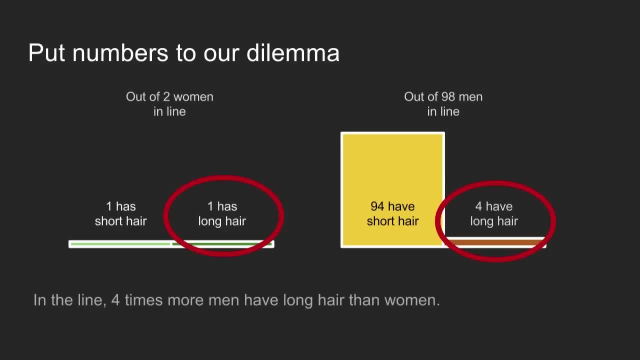 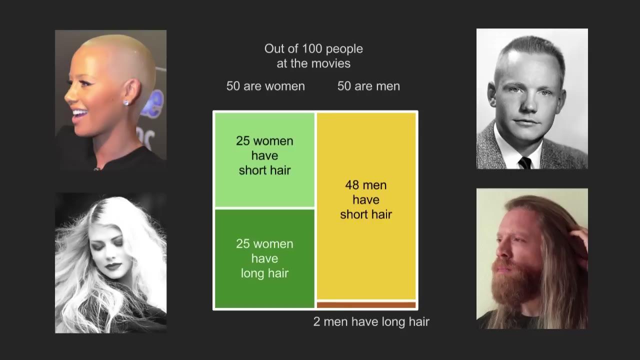 but now there are four times as many men with long hair than women with long hair in this group. Now the safe money is to bet that this person is a man. So to draw this a little differently, out of 100 people at the movies overall, we'll make this assumption. 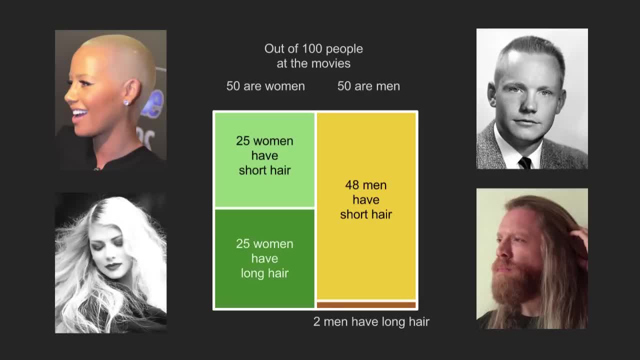 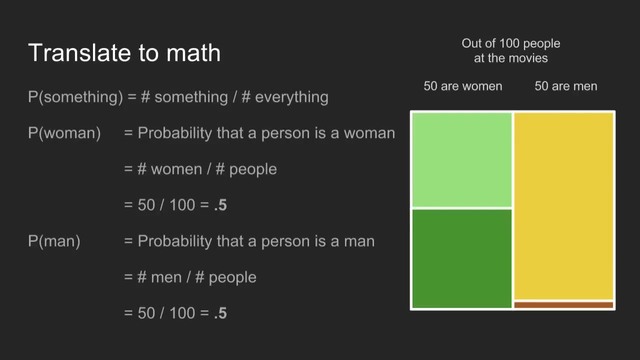 explicit that 50 of them are women, 50 of them are men. so this is how the different categories break down In the line for the men's restroom. then they break down a little differently. So to translate this to math, the probability that a person is a woman is the total number. 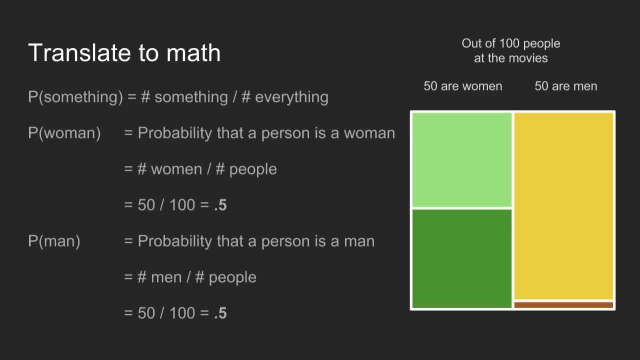 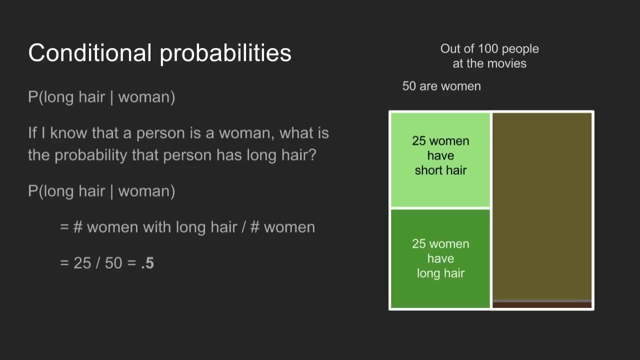 of women divided by the total number of people, 50%. similarly, for men Moving to the men's restroom line, the probability that someone is a woman is 2%- 98% for men. Now, Bayes' theorem is a little bit tricky, so to be very precise, 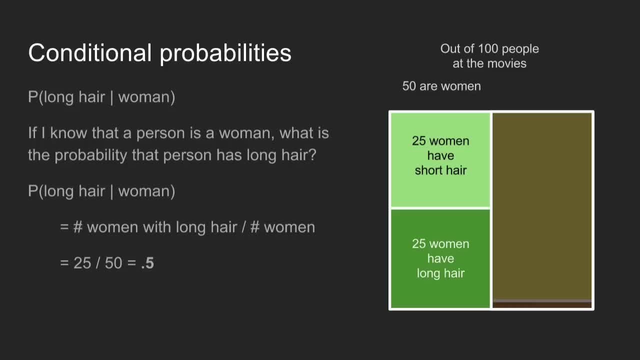 we're going to have to talk math. so if you bear with me, for just three probability concepts, we'll lay the foundation for presenting Bayes' theorem. The first one is conditional probabilities. If I know that a person is a woman, that's the condition. what's the probability that? 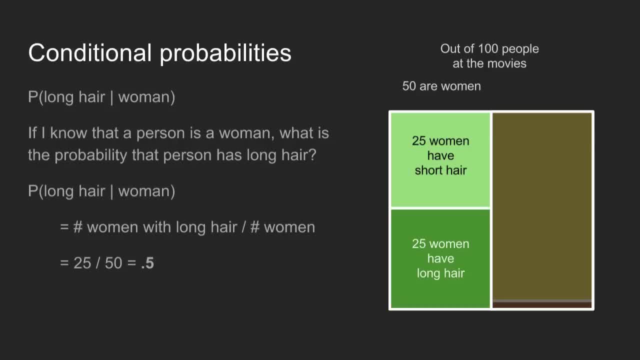 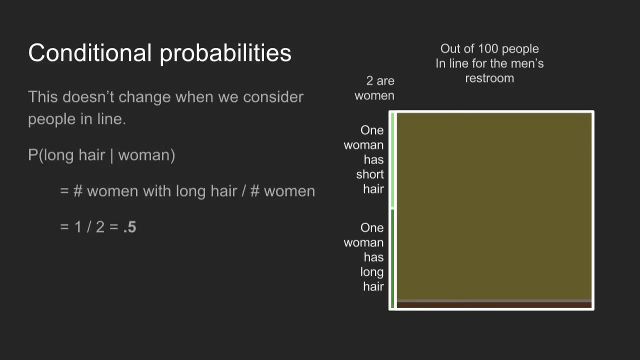 that person has long hair, So it's written as probability of long hair, given that a person's a woman. So to get this, we just divide the number of women with long hair by the total number of women- 50%, And this doesn't change whether there's 50 women in your group or 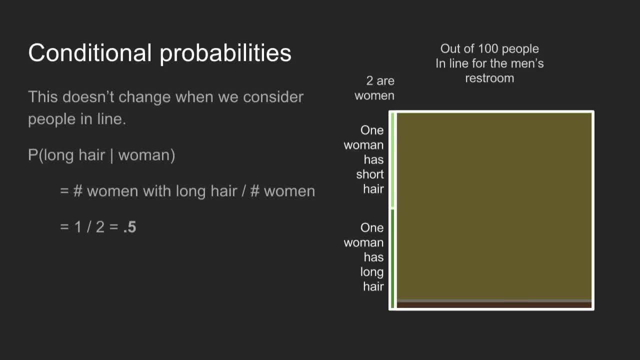 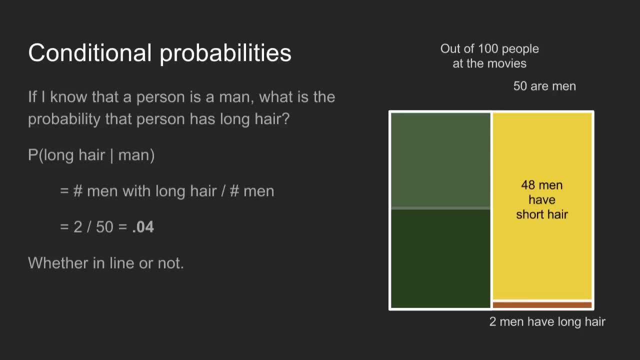 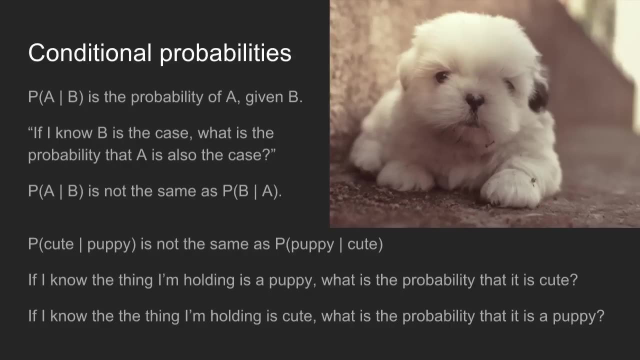 two women in the group. still, if we know that a person is a woman, the probability that they have long hair is 50%. We can do the same thing with men. Probability that someone has long hair given that they're a man is 4%. So conditional probabilities, if I know. 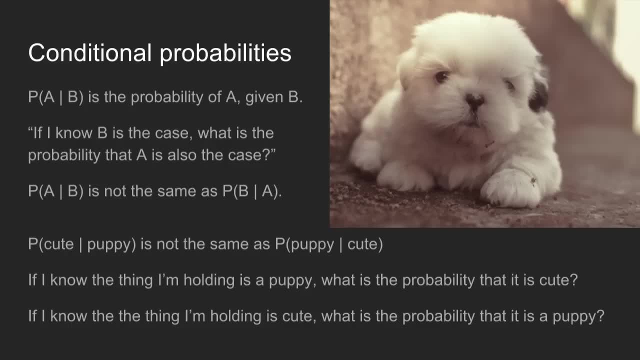 that B is the case, what's the probability that A is also the case? You can't reverse B and A and have this be true. So, for instance, if I know that the thing I'm holding is a puppy, what's the probability? 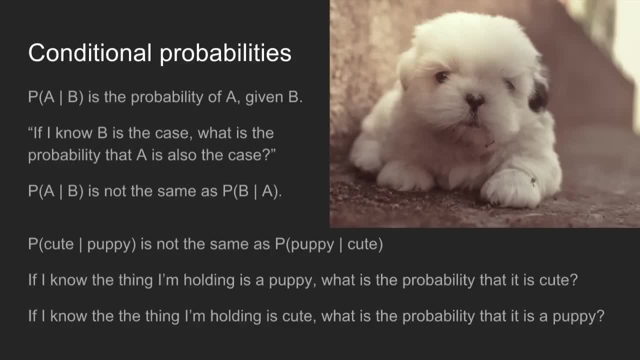 that it's cute. The probability is very high. If I know that the thing I'm holding is cute, what's the probability that it's a puppy? Well, it might be a puppy, it might be a kitten, it might be a hedgehog, it might be a small human. 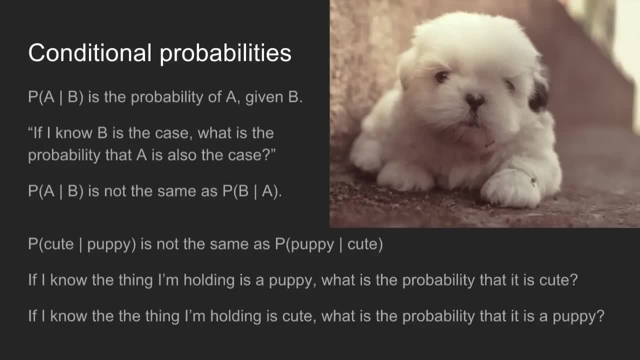 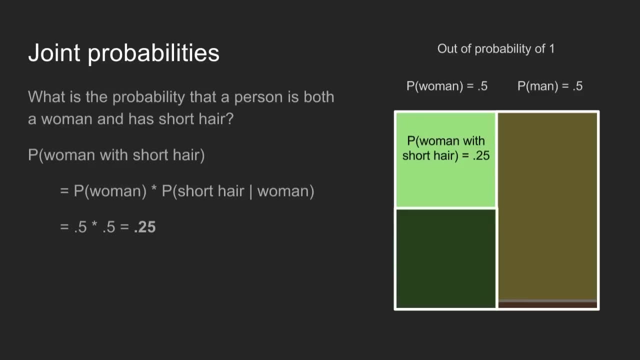 There's lots of things that it could be. So the probability there is less moderate. So these things are not interchangeable in conditional probabilities. Now concept two joint probabilities. So what's the probability that a person is both a woman and has short hair? So to calculate a joint probability you first find their conditional 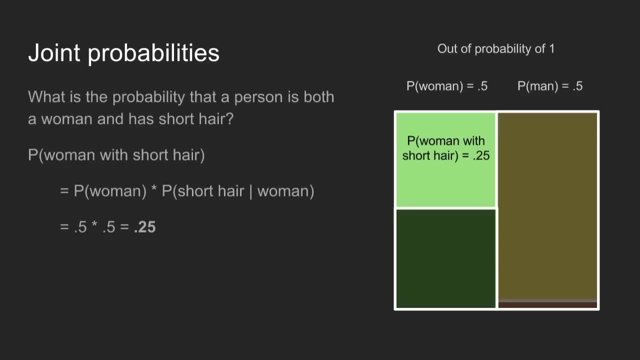 probability. Well, if I know that they're a woman, what's the probability that they have short hair? And then you multiply that by the probability that they're a woman. So in this case, 0.5 times 0.5, we get a 0.25, which is exactly what we knew it was going to be. 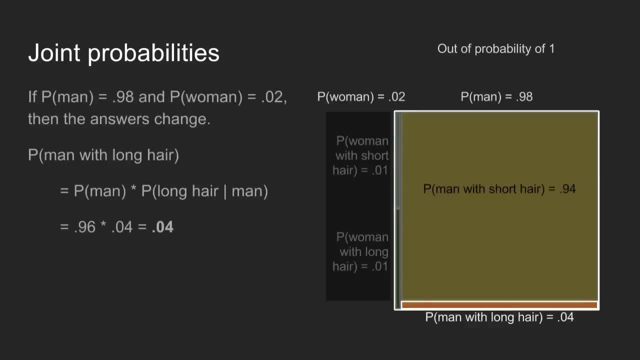 And the same is true for all of our different conditions, So we can do this for the men's restroom too. The probability that someone is a man and has long hair: 4%. Someone is a woman and has long hair: 1%. 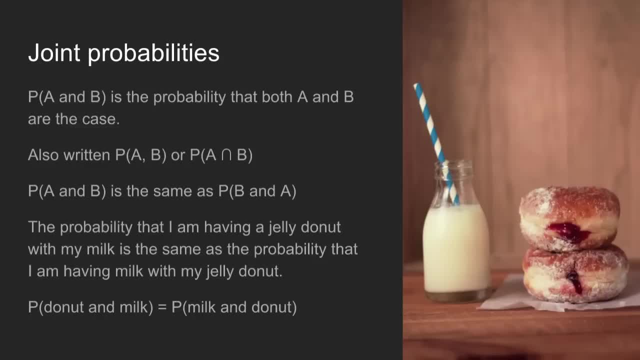 Joint probabilities are different than conditional probabilities. Here the probability that A and B is the case is the same that the probability that B and A is the case. So the probability that I'm having a jelly donut with my milk is the same as the probability that I'm having a milk with my jelly. 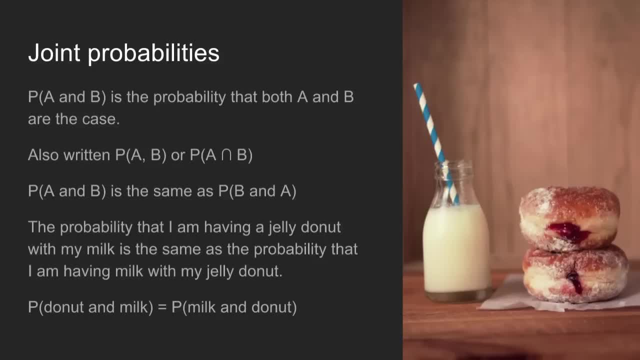 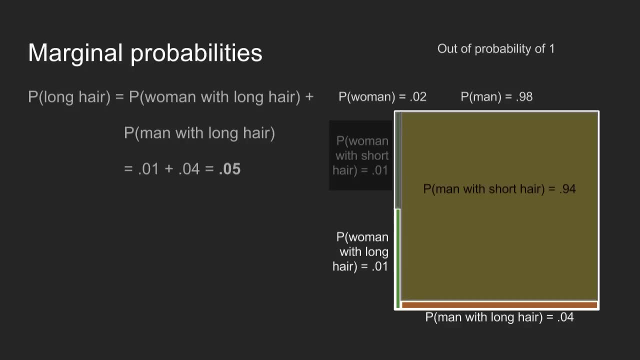 donut. These two conditions, these two situations are identical, So we can swap the order And finally, concept three marginal probabilities. If I wanted to say, figure out the probability that someone has long hair, I just add up all of the different ways that someone can. 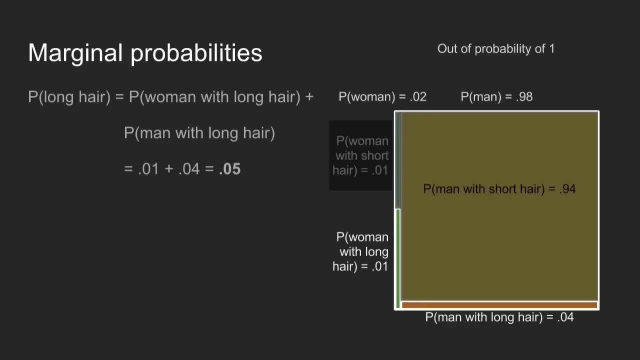 have long hair. They can be a woman with long hair or a man with long hair In the men's restroom line. that's a 1% probability plus a 4% probability, or a 5% probability overall, And you can do the same thing for short hair- 95%. Now this last concept finishes our foundation. We 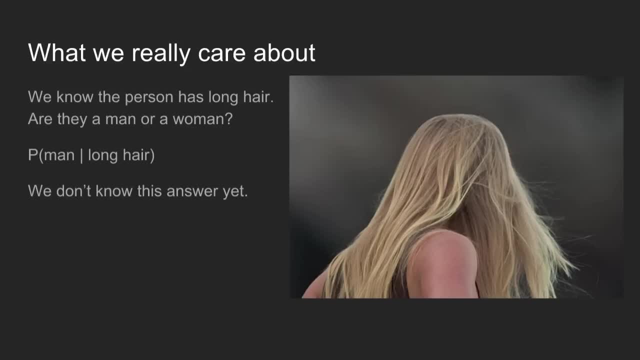 can get to what we really care about. We know that this person has long hair. What's the probability that they are a man or a woman? This is a conditional probability, but it's the reverse of the one that we know, And we don't know how to answer this yet. So this is where Thomas Bayes 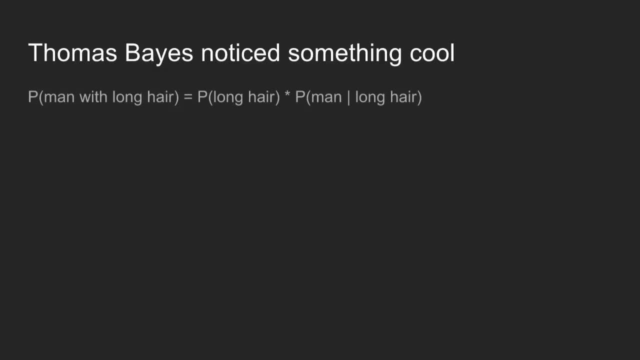 comes in, He noticed something really cool. You can calculate the joint probability that someone is a man and has long hair. You can calculate the joint probability that someone is a man and has long hair Using the formula we saw before, And you can also calculate the joint probability that someone 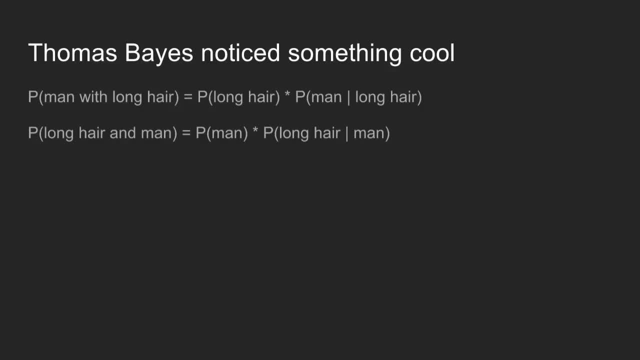 has long hair and is a man. Now, these are different formulas, but remember joint probabilities, don't care about the order. So these two things are equal, which means the stuff that they're equal to on the other side are also equal to each other. And we can do a little algebraic sleight of hand And now we have a. 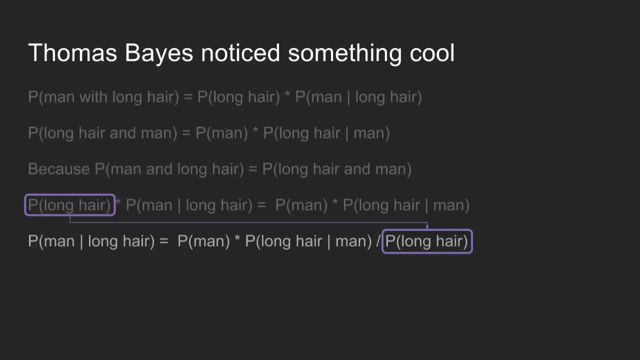 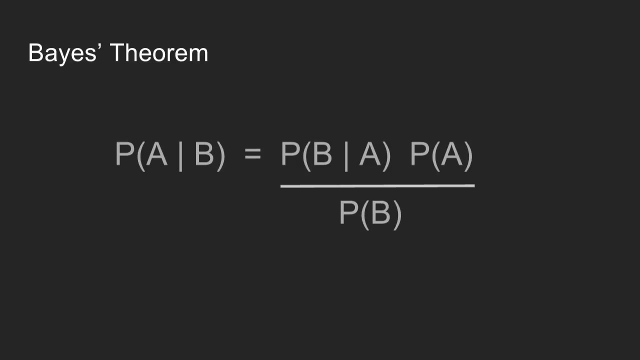 formula for what we want to know. If someone has long hair, what's the probability that they're a man? We have this expression to the right. We can genericize that with A's and B's, And now we have Bayes' theorem, One of the top 10 most popular math tattoos of all time. 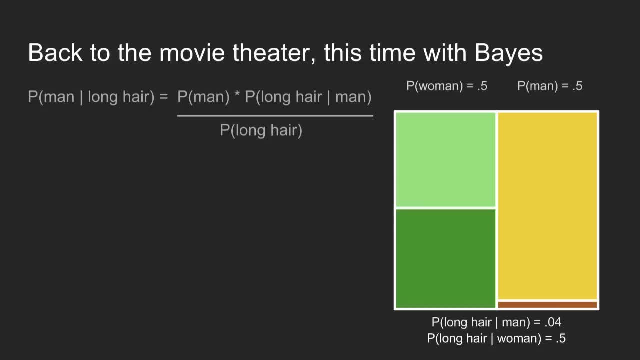 So, using this formula, we can go back to the movie theater and plug in what we know. We know that, the probability that someone is a man, We know the probability that, if they're a man, they have long hair, And we know the conditional probability or, sorry, the marginal probability that someone has. 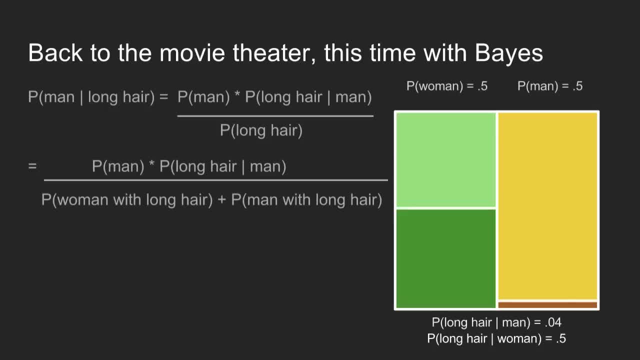 long hair, which is just the probability that someone's a woman with long hair plus the probability that someone's a man with long hair, And we plug all that in And we can say: if someone has long hair at the movie theaters, there is a 7% chance that they are a man. 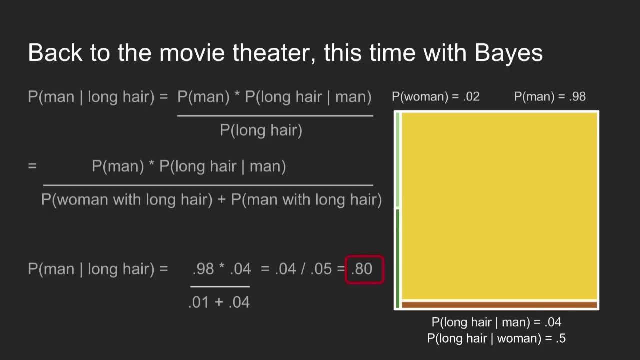 Similarly, 93% chance that they are a woman. Now, if they're in line for the men's restroom, because some of those probabilities change, that conditional probability changes. Someone's in line for the men's restroom and has long hair, there's an 80% chance. 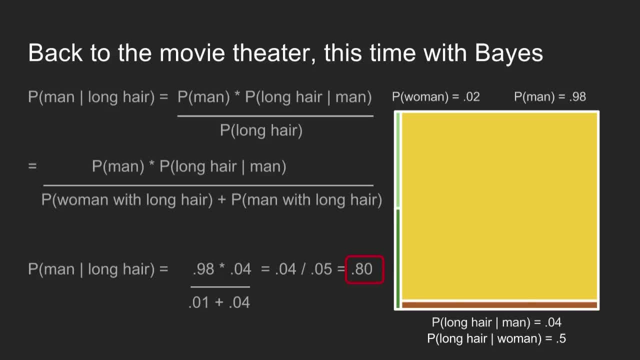 that they are a man And this is consistent with what we saw before. We know that there are four men and one woman for every hundred people in line for the men's restroom that have long hair. So four out of five long-haired people are men- 80% It all adds up. 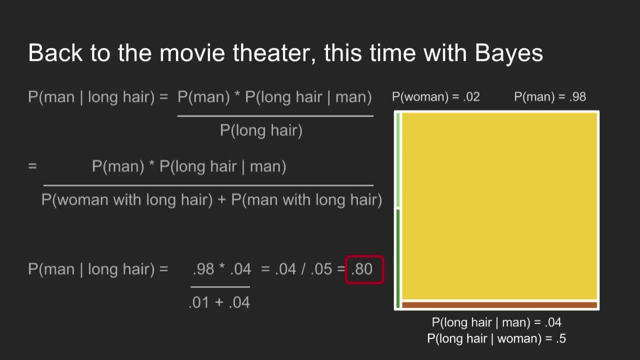 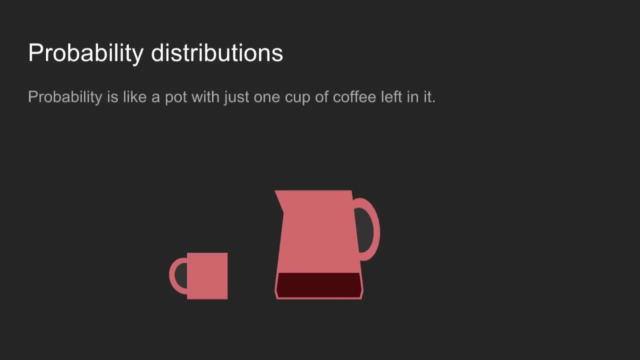 So this example shows the mechanics of how to get Bayes' theorem and how it works In practice. it's usually used a little differently, So to show this we'll have to do a little bit of a detour and first talk about probability distributions. 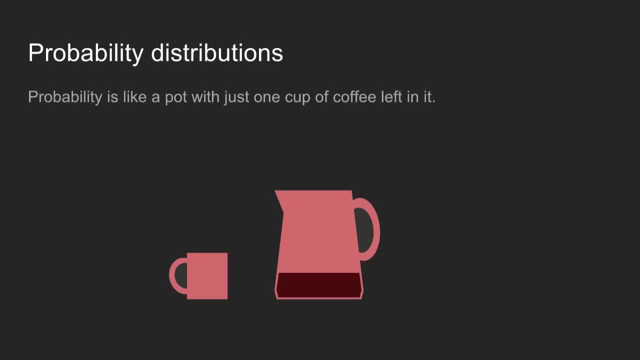 Probability. you can think of probability like a pot. with just one cup of coffee in it, You can fill up. if you just have one cup to fill up, you can fill it all the way to the top. But if you have more than one cup you have to share it around, or? 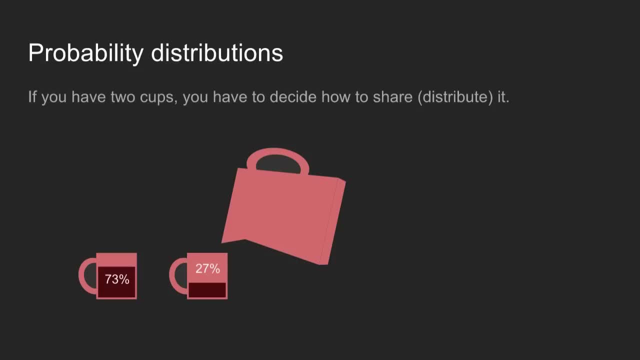 distribute it And you can share it with any proportion you want. So, for instance, if we're representing the number of men and women at the movies, we could share it 50-50, but it'll always add up to 100%. We could even share it further into. 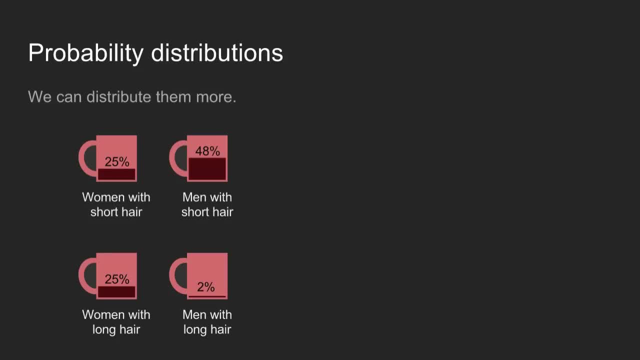 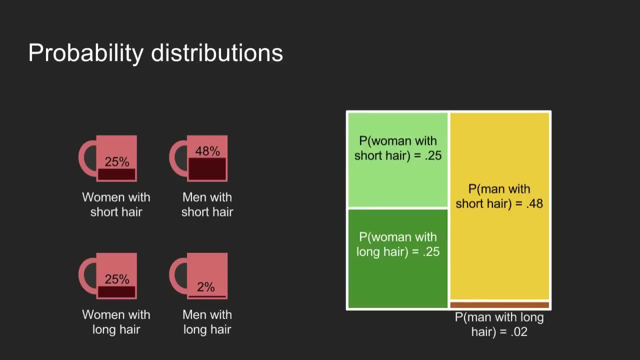 different categories. So here we see the joint probabilities of all of our four different categories that we were working with, And you can see that this is just another representation of the distribution representation that we were looking at before Now. usually when we look at this they're side by side. 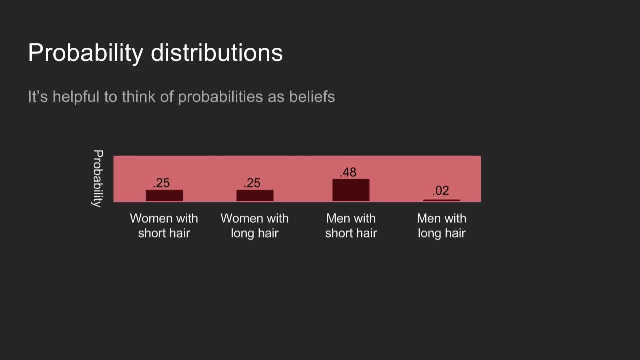 probability instead of percentage and shown in a histogram like this, It can be really helpful to think of these as beliefs. So, for instance, if I flip a coin and hide the result from you, you might half believe its heads and half believe its tails, until I tell you what it is. If I roll a die and hide the result from, 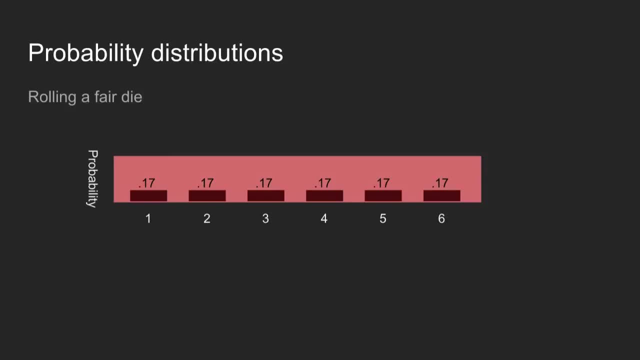 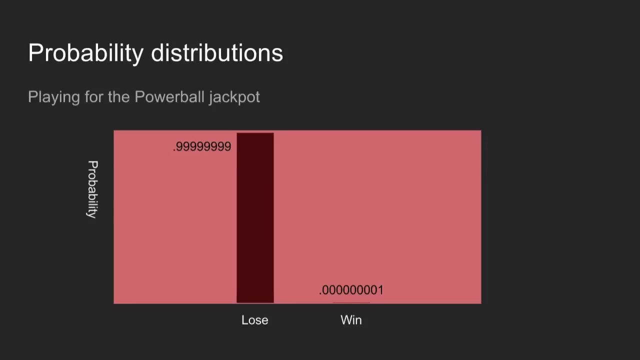 you. you might believe about one-sixth, that it's a one or a two or three or four or five or six, Until I show you the result. So these are what you believe. Probabilities can represent what you believe about something before you measure it. Similarly, 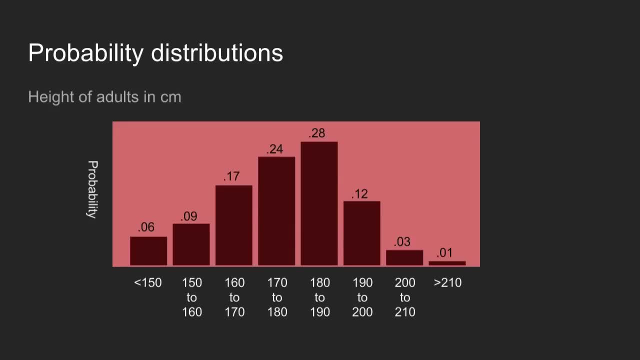 for Powerball tickets and even for things that are more complicated, like, let's say, the height of adults in the United States in centimeters. You might believe that there's a very small chance that they'll be over 210 centimeters and a smallish chance that they're really small. 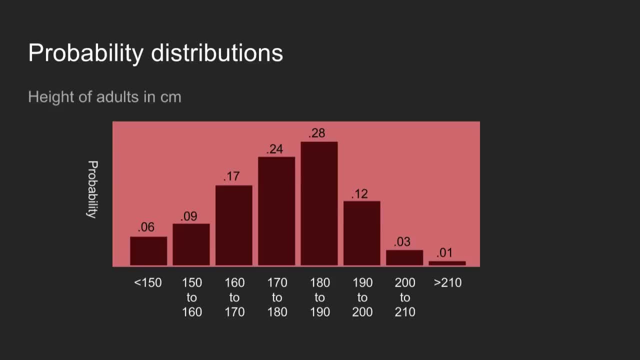 There's a chance that they're less than 150 centimeters, And then assign various amounts of this belief to all of the ranges in between, It still adds up to one. It's like all a bunch of cups of coffee lined up in a row and you put a. 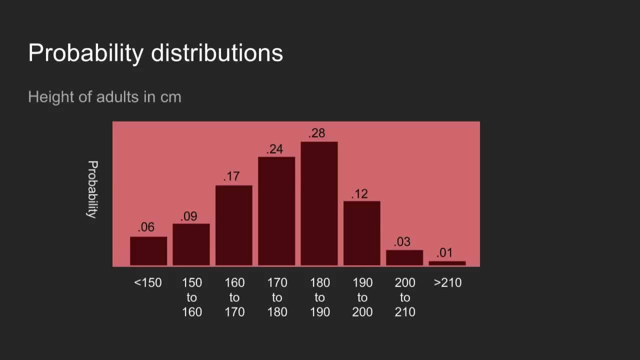 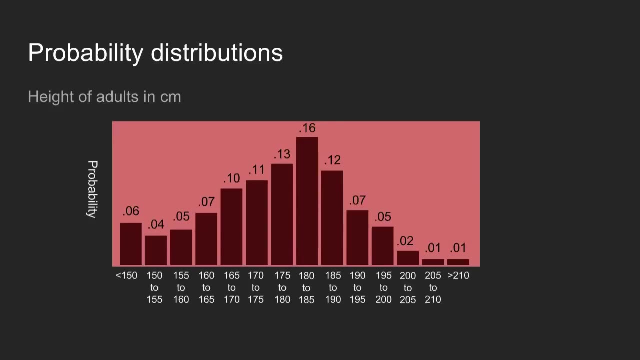 little bit in each one. The cups in the middle have more, And it shows how your belief about some individual is distributed, before you actually measured them. Now you can take these bins And chop them more and more finely, Again and again, And if you keep doing this, you 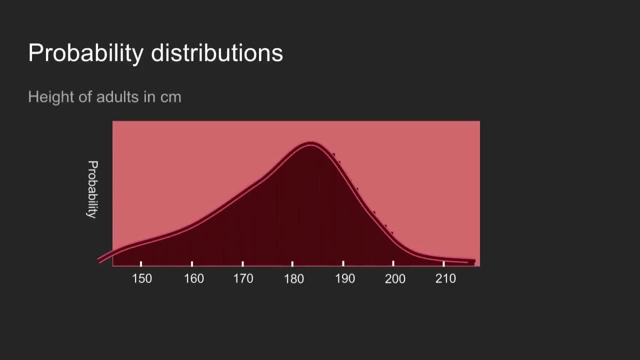 can get to something that's actually perfectly smooth. So it's as if you had an infinite number of very tiny cups and you put a tiny bit infinitesimal amount of coffee in each one. At this point it's probably no longer helpful to think of it in that terms, But 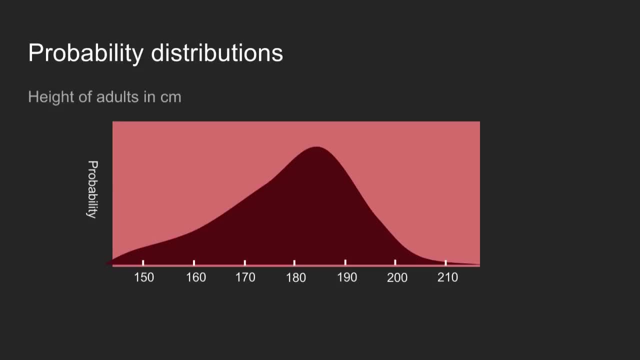 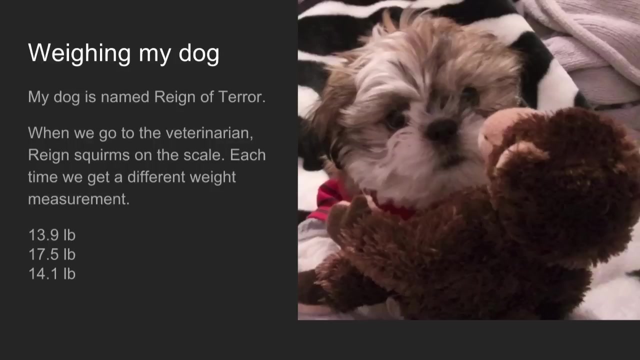 just thinking of it as a continuous distribution showing for all these high heights. Where am I placing my bets? What do I believe And how much? So, once you have your beliefs, you can use it to answer questions about typical heights, The average, the median value, the most common value or the mode. Now we'll 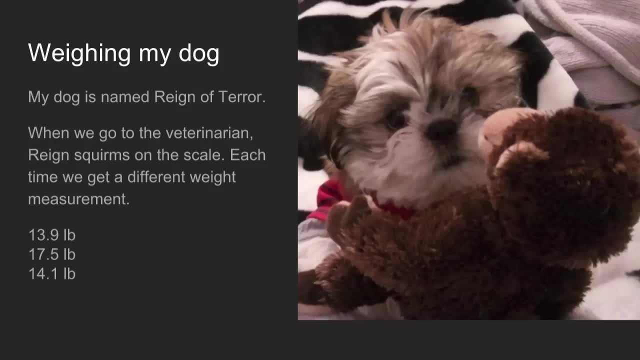 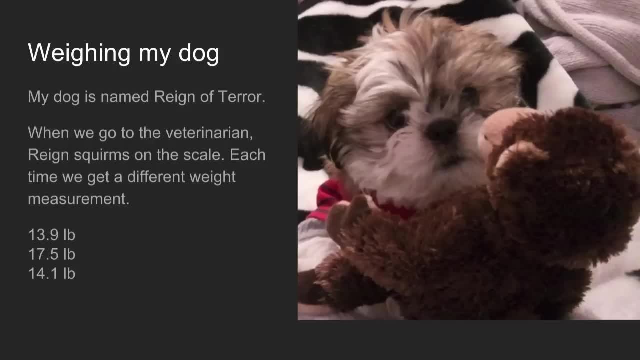 she's a little mischievous, And when we go to the vet she's a little mischievous, And when we go to the vet she's a little mischievous, And when we go to the vet and death. so we don't want to make the wrong assumption and draw the wrong conclusion. 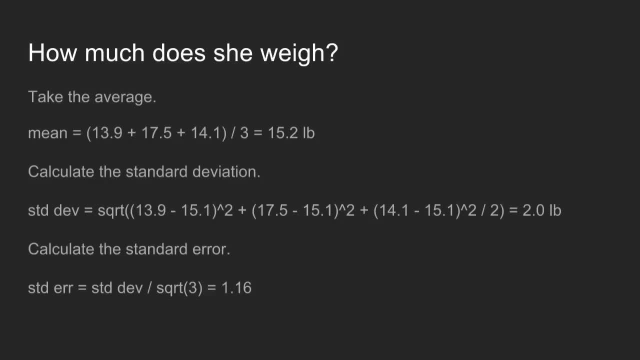 so if you've ever taken a statistics class before, you know you can take these measurements. add them up, get the average 15.2 pounds. you can calculate the standard deviation of these three measurements and also the standard error and come up with a 1.16 pound standard error which, when you show, 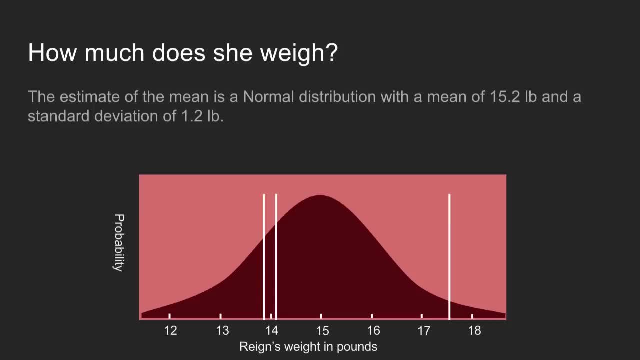 it graphically. this red curve now shows the belief that results from those three measurements. the distribution, the peak of that hill is at 15.2 pounds and one standard deviation on that curve is our standard error of 1.2 pounds. so you can see, looking at this, that yes. 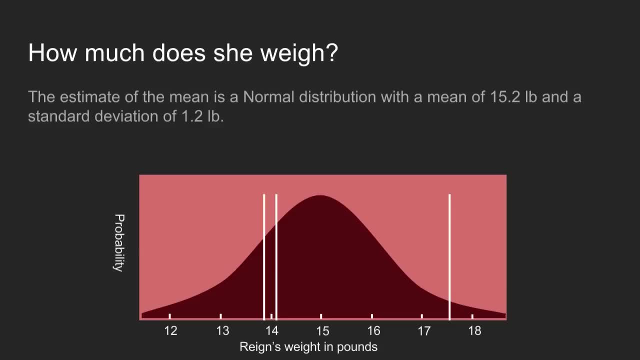 it's most likely that she's 15.2 pounds, but there's a lot of that curve that sits out of the picture and that's what we're going to be looking at here. so we're going to be looking at outside of the range of 14 to 16.. so, yeah, she's probably between 14 and 16 pounds. 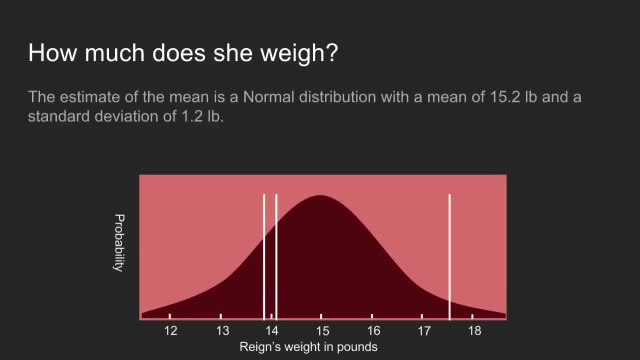 most likely between 13 and 17 pounds, but she might even be lower than 12 and higher than 18.. that is a really wide range and it's not a great basis for making a decision now. you can see the three measurements there, those three white vertical lines, and you can see why our belief. 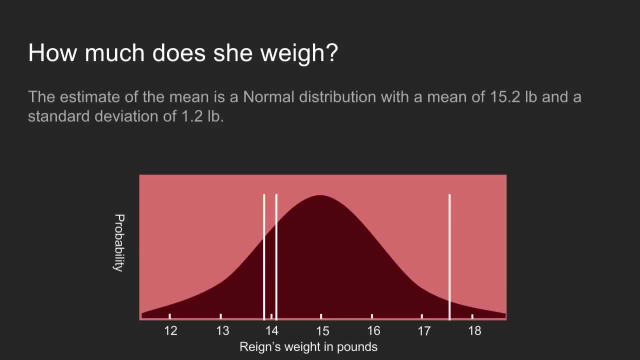 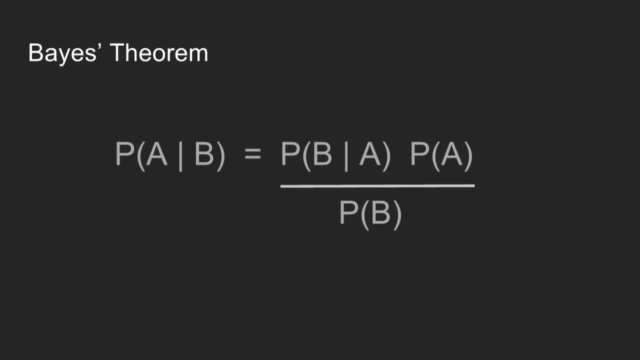 is so district, uh, dispersed, because those three measurements are pretty dispersed, it's hard to capture all that in one distribution, so let's try it again with bay's theorem. so the way we'll do this is, instead of a and b we'll substitute in w for her actual weight. 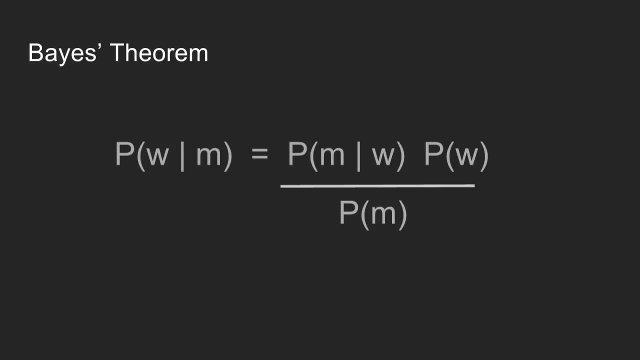 and m for the measurements that we took now this term over here. the probability distribution of the actual weight is our prior. this is what we believe about her weight before we put her on the scale. the probability given a weight of getting certain measurements are the likelihood associated with those measurements. 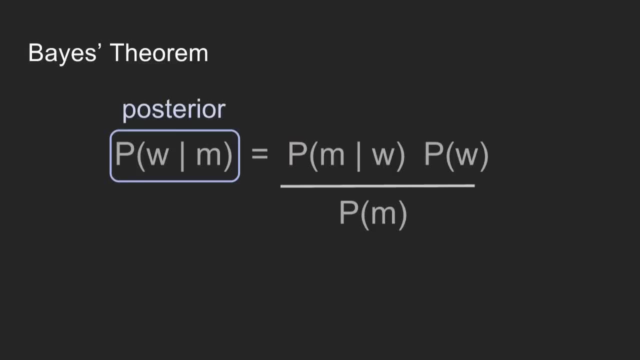 and then the posterior is what we believe about her weight, given those measurements. so you can think of this as we start with a belief, we take some measurements and we update it, and then we have a new belief when we're done. this term on the bottom we're going to ignore. 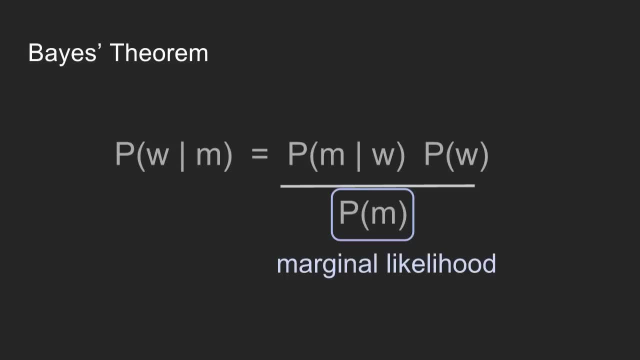 for the most part it'll be a constant, but it's called the marginal likelihood, so we're going to start by not assuming anything about. her weight could be one pound, 10 pounds, 20 pounds, 100 pounds. we're going to let this be uniform and we're going to 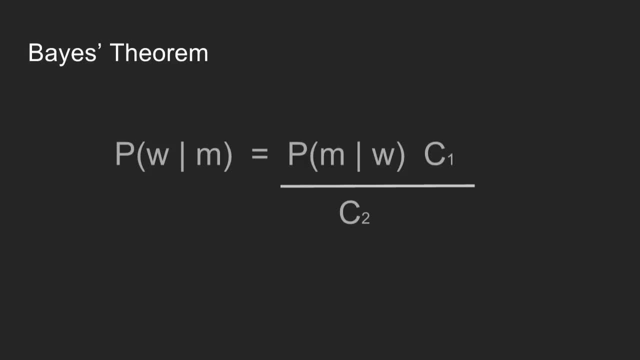 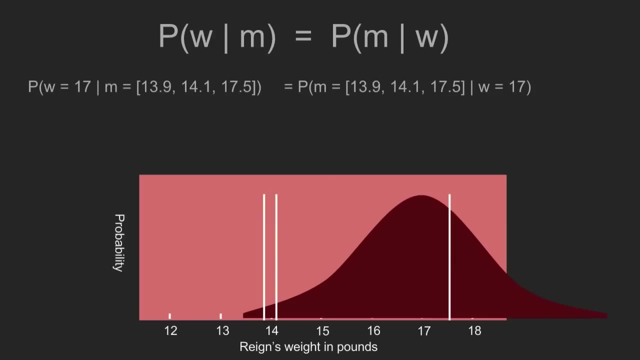 let the data speak. so now our formula looks like this. we can further simplify it, and so we want to calculate this. we want to calculate the probability of our measurements occurring given a weight, and we want to do this for all of the possible weights, and then we'll. 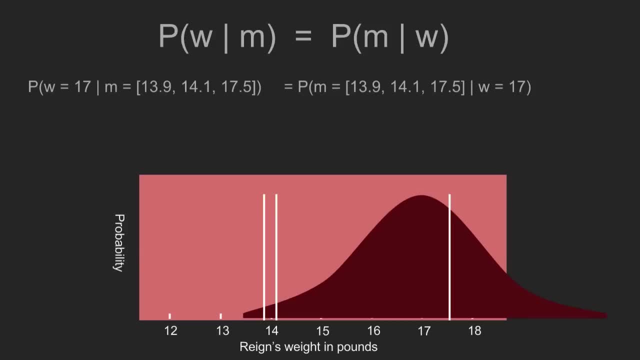 end up with a new distribution, which is our belief. what's the probability of each of those weights occurring, given the measurements? so these two things are identical. so let's start, for instance, by assuming what if she weighed 17 pounds in reality? now, because our measurement process is 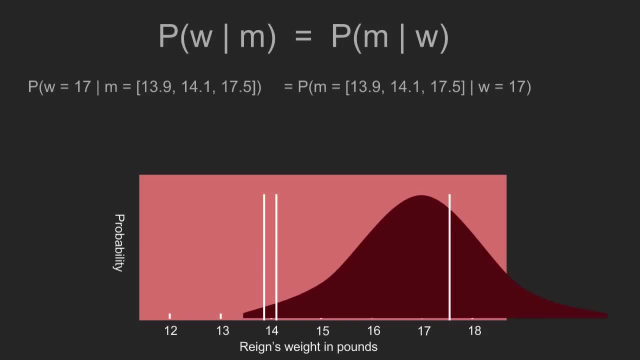 very noisy, as we saw. if she weighed 17 pounds, we would expect those measurements to be distributed as shown here. some would be up way above 18 pounds. someone would be down around 14 pounds where we actually measured, but not very much, and so we want to start by doing some kindergarten now. what we'll be doing in this training es. this is a lot of measuring amounts. after some of 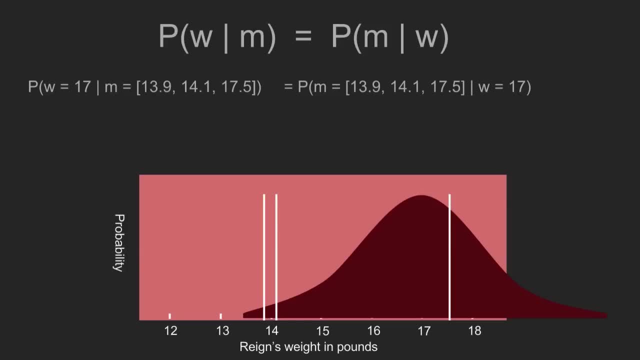 you will take some encouragement to figure out what weight is actually expected as you begin with the measurements and finally we measure. very many of them would be. So to calculate now the probability of our measurements occurring given this weight, we find what the probability of each individual weight is of occurring. 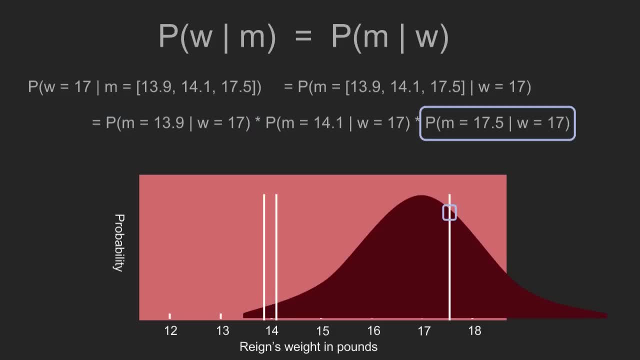 and we multiply that times, that times that Now these two are pretty small. When you multiply two small things together, they make something very small. So the probability of her being at 17 pounds is pretty small. We shift our belief over and say, well, what if she was 16 and a half? 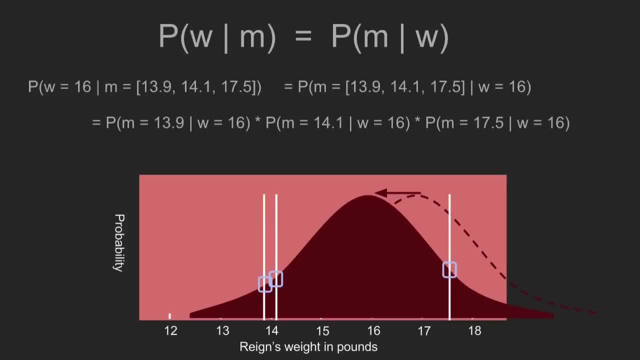 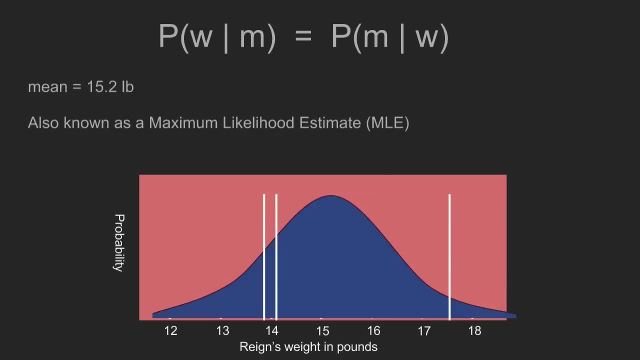 pounds- What if she was 16 pounds? And we recalculate it each time, multiplying all of those actual probabilities together, And then, by the time we're done, this is what we've measured at each of those weights, This is the likelihood of each of those occurring, And you can see that. 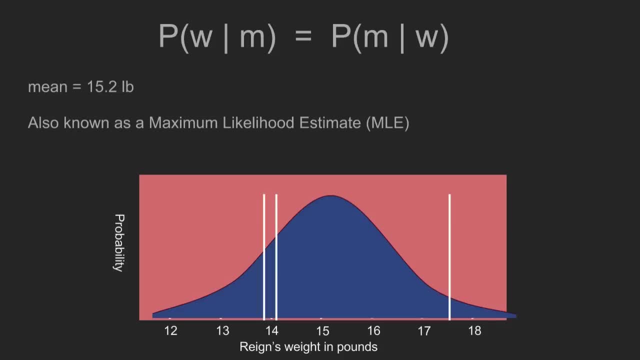 the maximum likelihood occurs at 15.2 pounds, And this is commonly called the maximum likelihood estimate, where you start with a uniform assumptions on your weight, And it just so happens that the standard error on this is exactly what we calculated before. A very cool thing, connection. 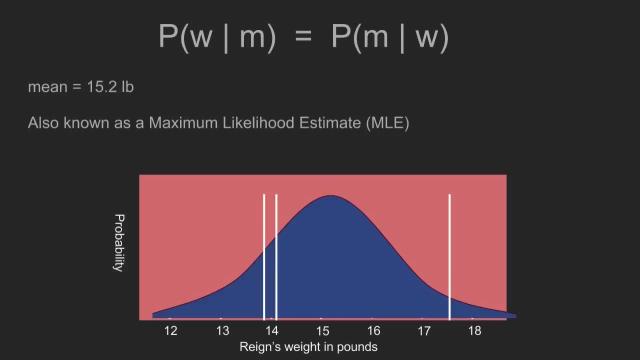 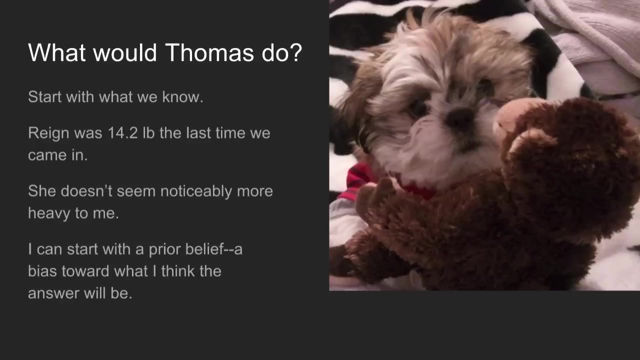 here, When you take the average and calculate standard deviation and standard error, it gives you the likelihood that you would get by doing Bayes method and assuming a uniform prior, not assuming anything about what the results going to be. So we've already established, though, that that's a really broad result and not helpful. So we 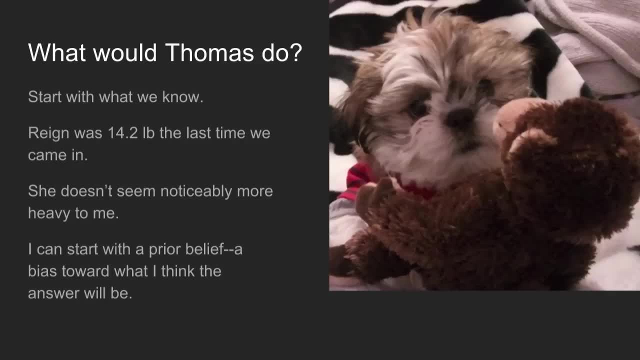 need to start over now and let's start with what we know. So some background information. Rain was 14.2 pounds The last time we went into the vet And she doesn't seem noticeably more heavy to me. My arm is not that well calibrated, but let's, I'm going to. 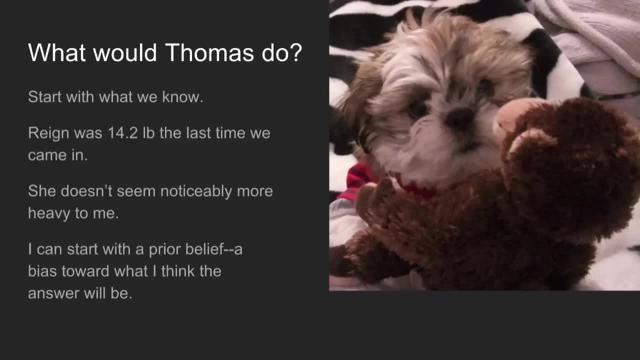 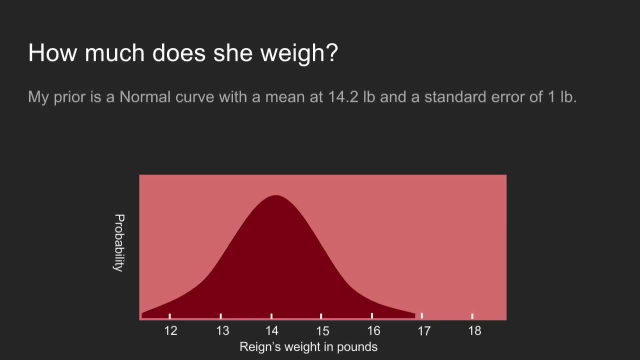 assume that she's within about a pound of where she was before. So I take that prior and this is the form that it takes: A normal distribution centered on 14.2 pounds And you can see that most of that bulk is within plus or minus a pound And it extends a little bit further out. I allow for the possibility that she's. 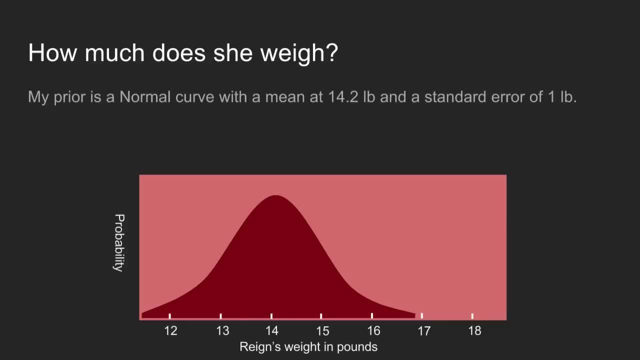 actually gained a lot or or a lot of weight, Lost a lot of weight, but probably she's pretty close. This is what I believe before I even put her on the scale. This is the probability, the prior the probability of her being a given weight. 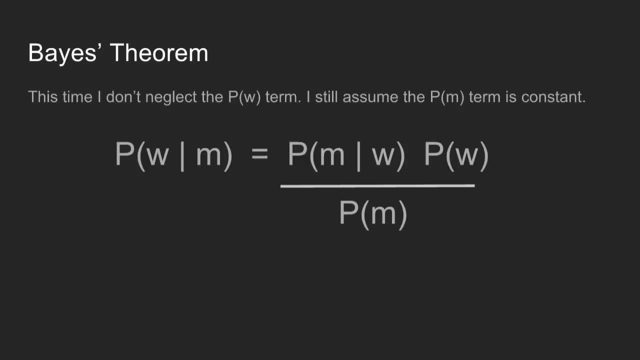 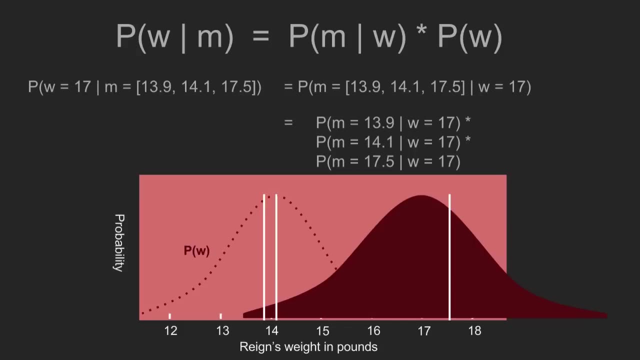 So this time we're not neglecting the prior term, We're not setting it constant, We're going to use it. And the way this plays out now is: we assume: okay, what if she were 17? 17 pounds, like? well, we need to multiply that now by the probability of our prior showing that she's 17. 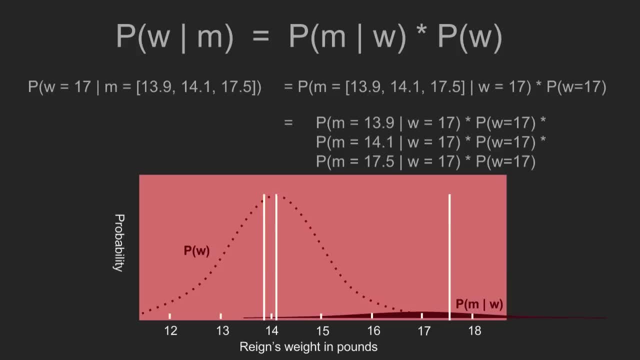 pounds, which actually makes that quite small. Now we calculate and multiply the three probabilities of our measurements occurring. So now we have something small times something very small times something very small. So we get a very small result, a probability that she will act, that she actually weighs 17.5 pounds. 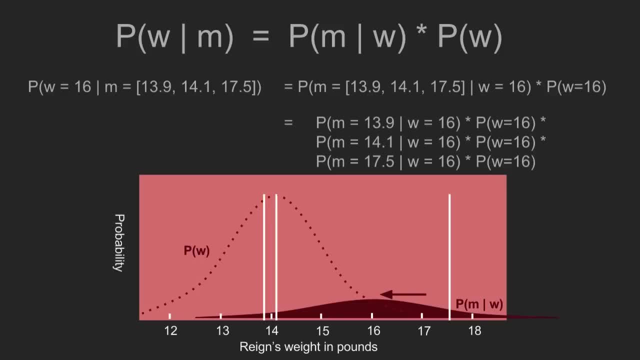 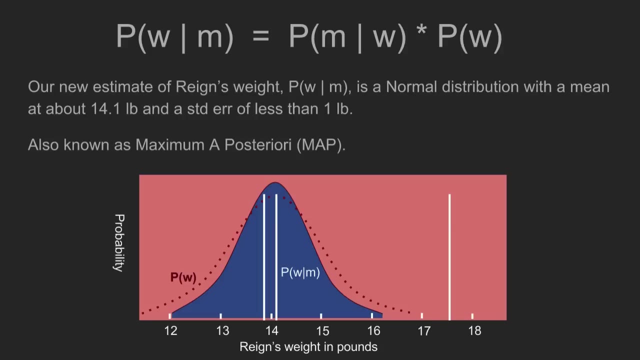 17 pounds, And now we repeat this process at 16 and a half pounds, and 16 pounds, and 15 and a half pounds, and 15 pounds all the way through, And then, by the time we're done, we tally up all of those and we get this new posterior distribution. 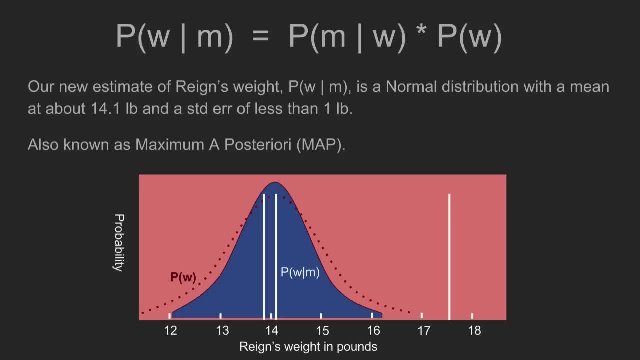 It's normally distributed at about 14.1 pounds and it has a standard error of less than a pound. You'll notice it's even narrower. It's even narrower. It's even narrower than our original prior. So we've taken our original belief and we've been able to sharpen it up just a bit. 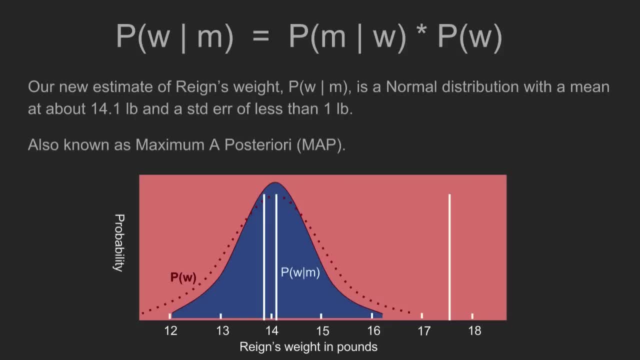 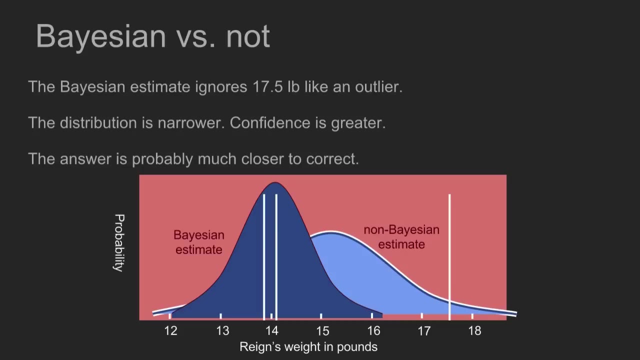 And so, incidentally, the peak of this curve is called the maximum a posteriori result. If we had to choose one value to represent our belief, that's not a bad one to choose. And now we compare this with our original estimate. It's labeled non-Bayesian here, but more accurately it could be non-Bayesian. 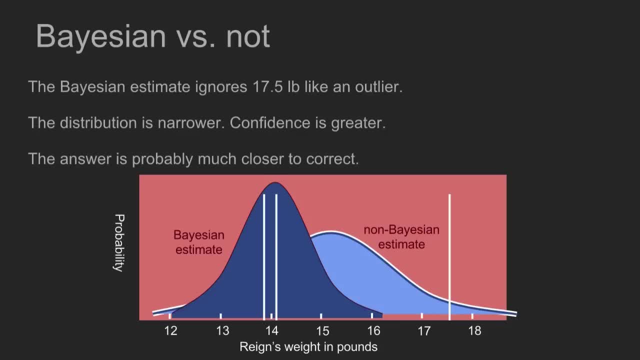 Bayesian with a uniform prior, You can see that it is much broader and also the peak of that curve is in an entirely different place. So the answer that we got: it's more confident because it's more centered and it's probably based on what we know closer to being correct. 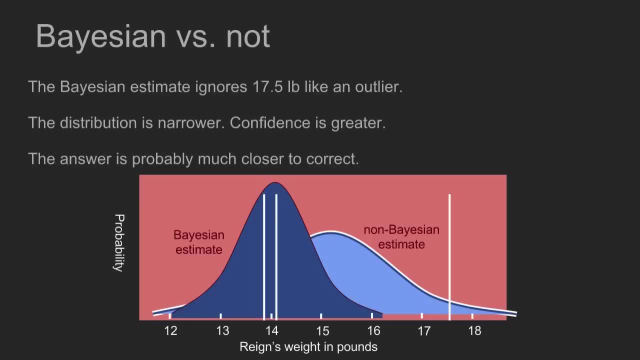 So this is how Bayes' theorem is used most often in data science or in analysis. So this is how Bayes' theorem is used most often in data science or in analysis. So this is how Bayes' theorem is used most often in data science or in analysis. 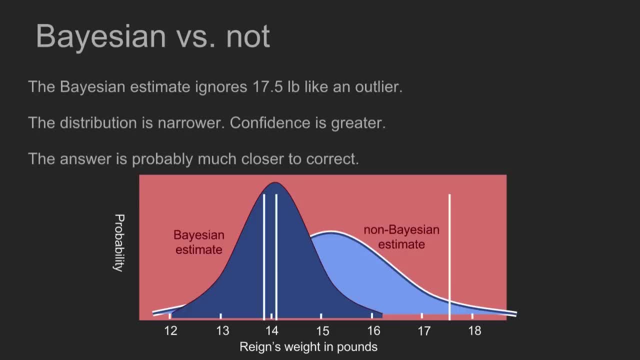 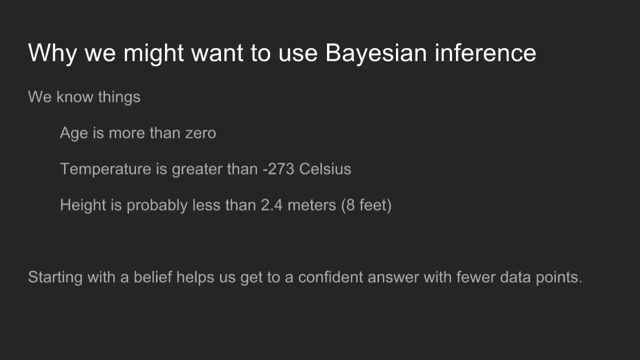 It's a prior that you then update, based on your measurements, to sharpen up and get a revised set of beliefs. So there's a lot of times that it makes sense to use Bayesian inference. Sometimes we just know things Like: if we're measuring age, we know that everyone is more than zero years old. 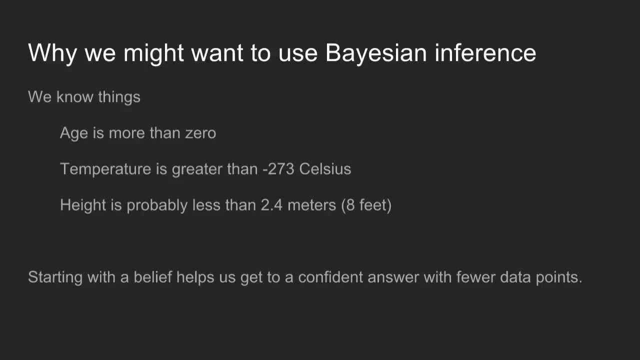 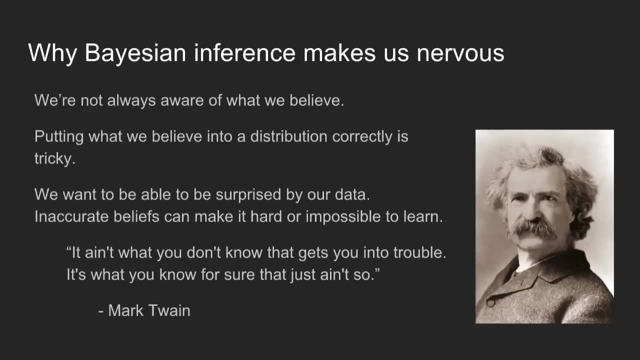 And so we can take that information and build it in And we can get sharper estimates with fewer measurements. Now it should, if you're paying attention, make you a little bit nervous. We humans are actually not always aware of what we believe. 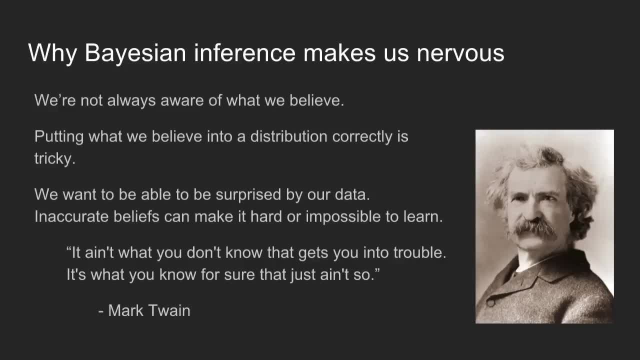 And putting it into a mathematical distribution can be very tricky. More importantly, the reason we're measuring something is because we want to learn about it. We want to know what's going on. We want to know what's going on to be able to be surprised by our data. So if we believe something that's not true, it can make it.